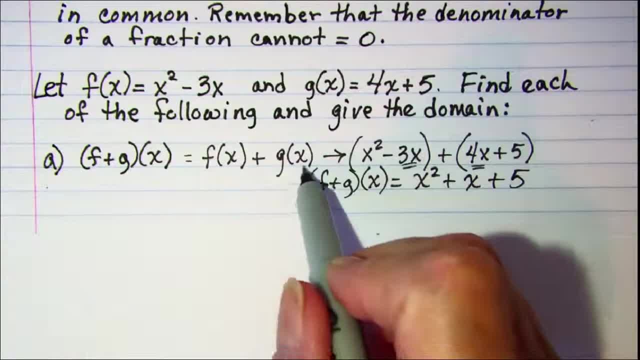 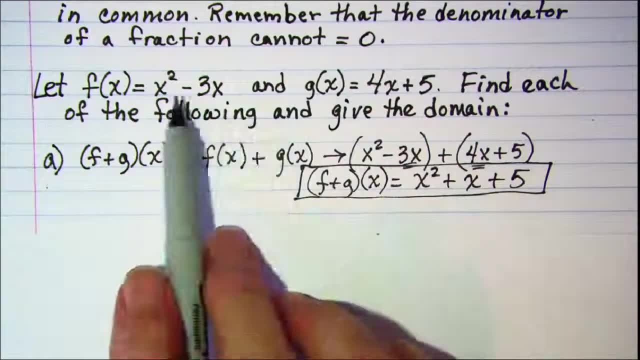 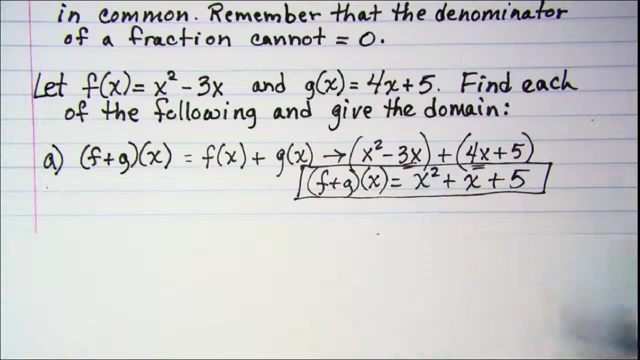 f plus g of x is x squared, and then we get x squared minus 5.. Now we'll look at the domain of f and f of x. Since there's no restrictions on the domain of f or the domain of g, then the domain of the sum of the two functions will just be all real numbers. 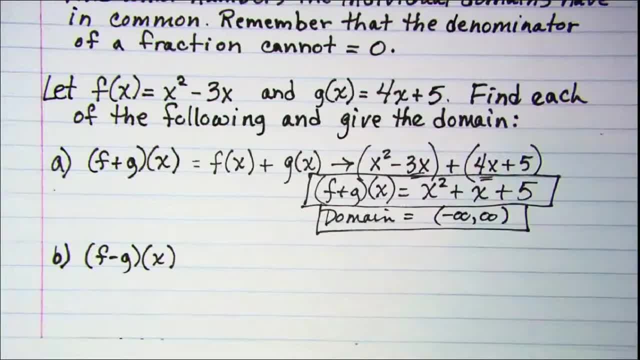 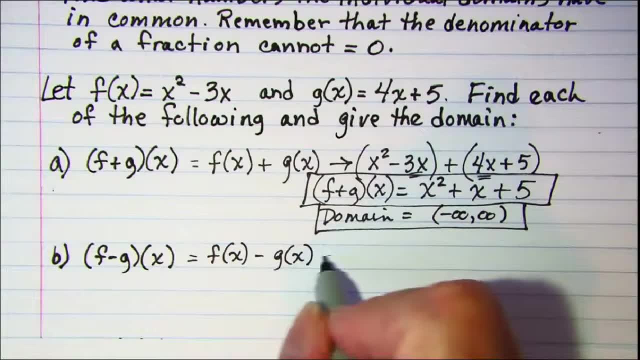 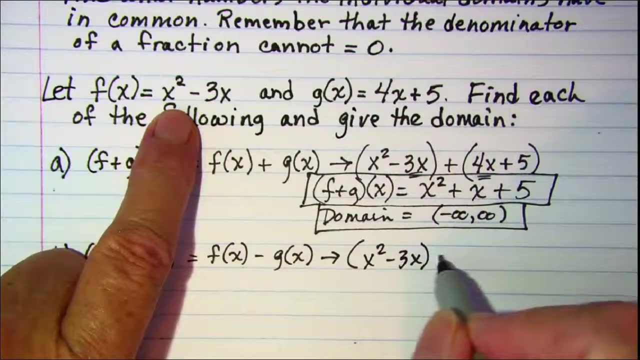 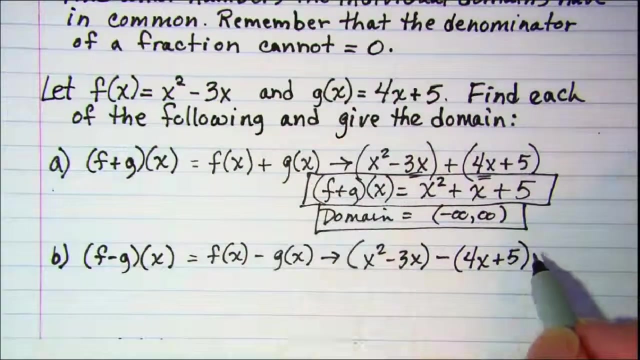 Next, let's look at f minus g. Again, that's equal to f of x minus g of x. So we have f of x, which is x squared minus 3x, subtract g of x, which is 4x plus 5.. Now in this one we'll need to distribute our negative 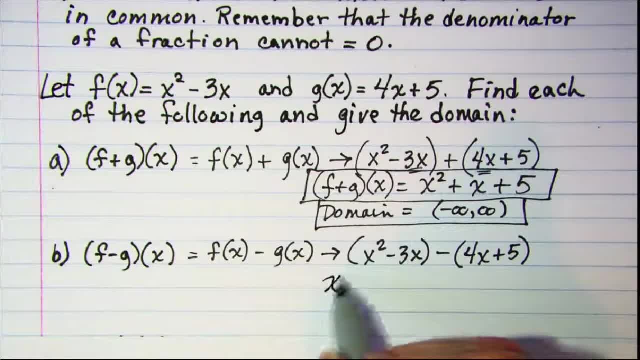 So this is x squared minus 3x minus 4x minus 5, so our difference is x squared and then negative 3x and negative 4x is negative 7x minus 5.. The domain again is still all real numbers. 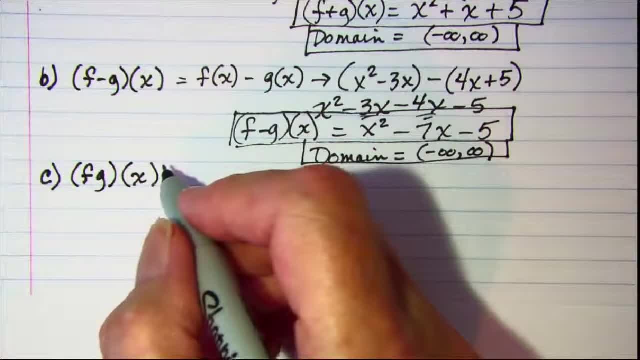 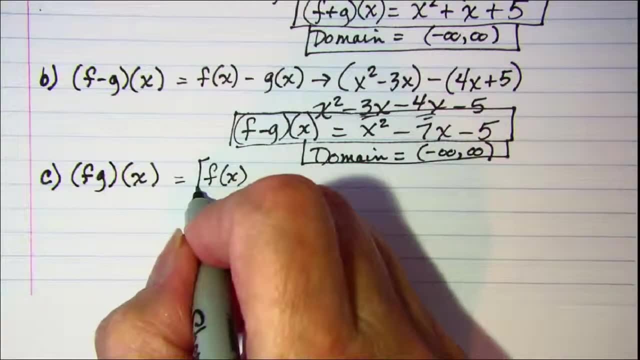 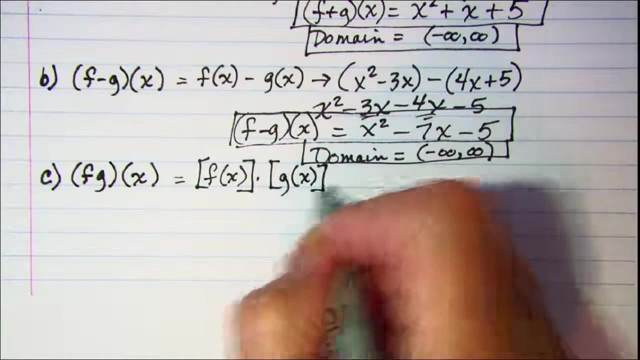 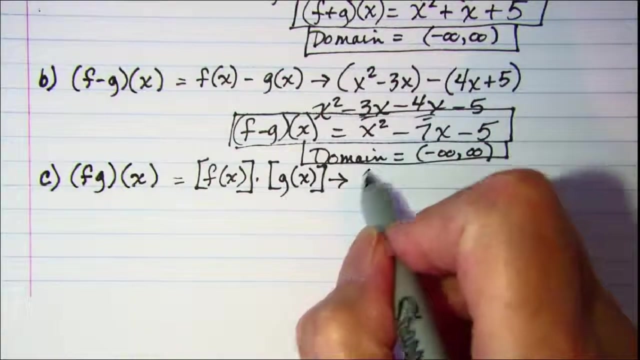 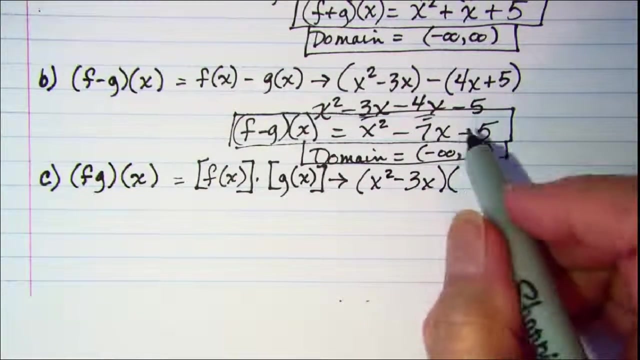 Next we'll find the product f times g of x, and that'll be f of x multiplied by g of x. Now f of x was x squared minus 3x, and then we're multiplying that by g of x, which is 4x plus 5.. 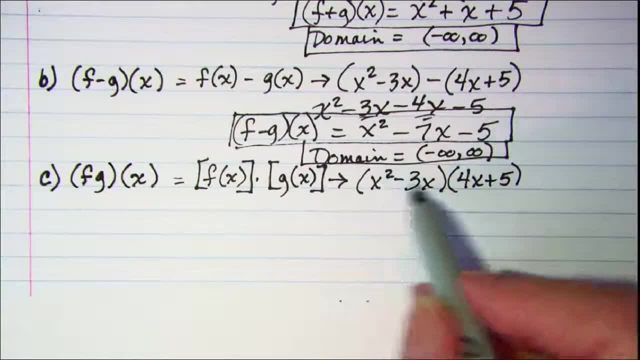 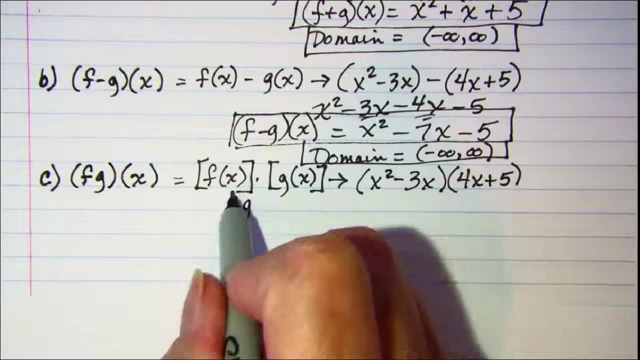 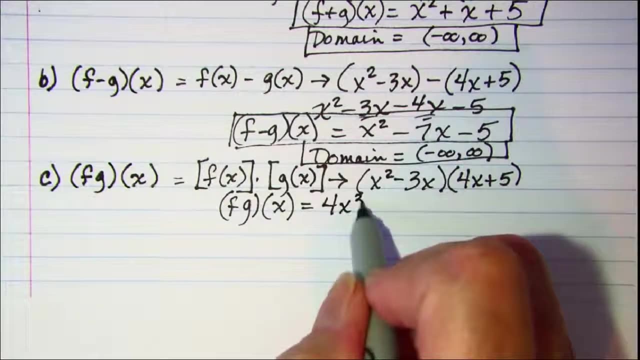 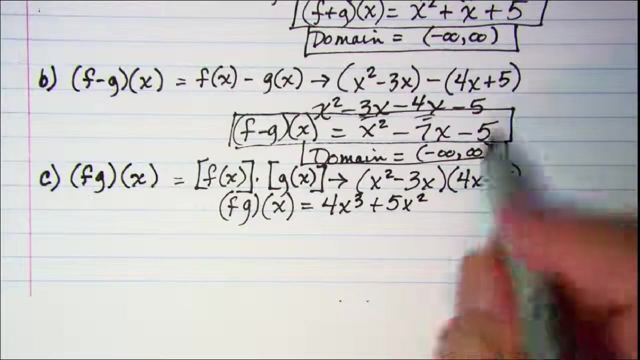 We'll use FOIL on this. so x squared times 4x is 5.. Next we'll take the third product for x, cubed, and then the outer product is x squared times five, and then the inner product is negative 3x times 4x. 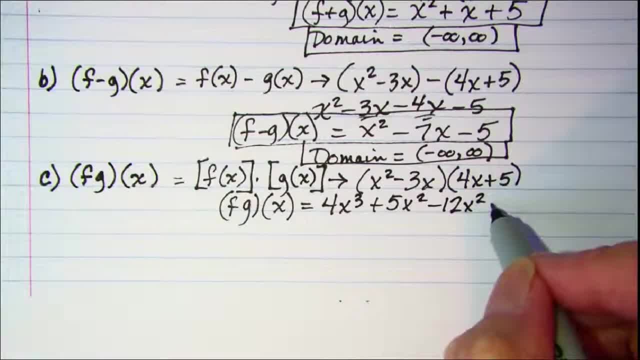 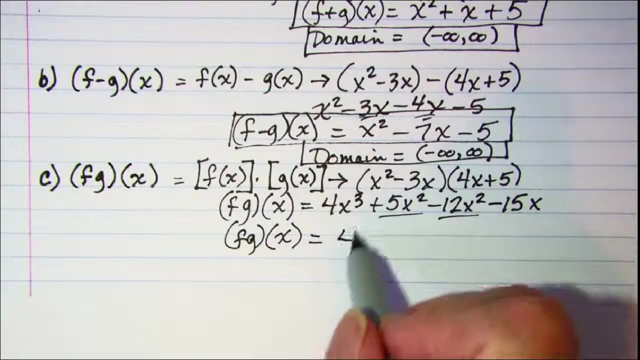 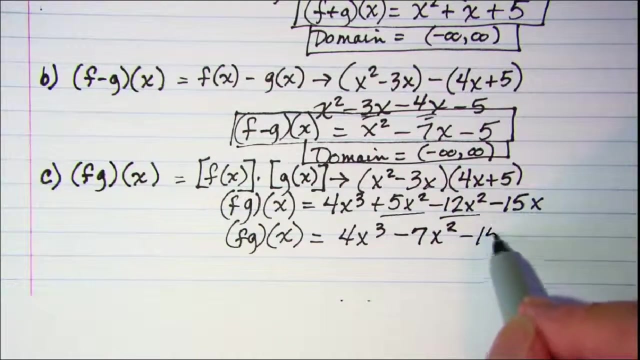 plus x, Then the last one's multiplied together- data 10 times three. and and then the last ones multiplied together 4x plus five and give me a negative 15x. We can combine these two, so f times g of x is 4x cubed, the negative 7x squared and then minus 15x. Again. no restrictions on. 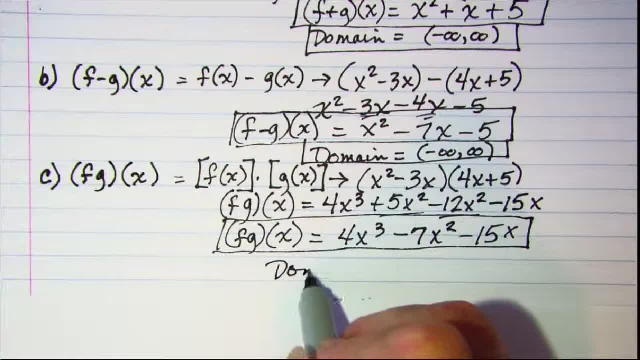 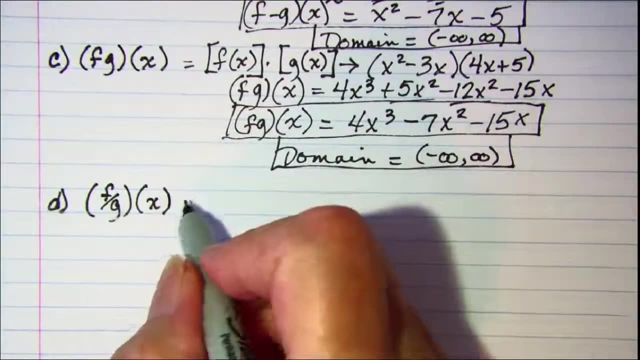 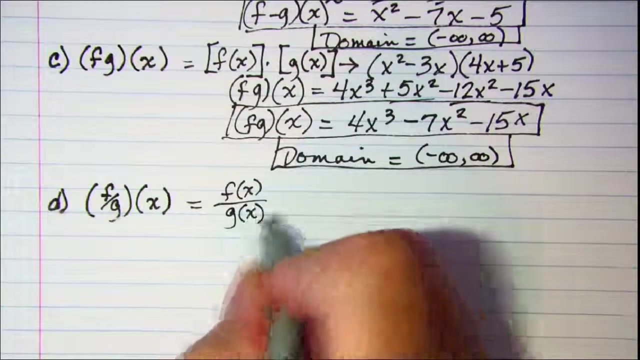 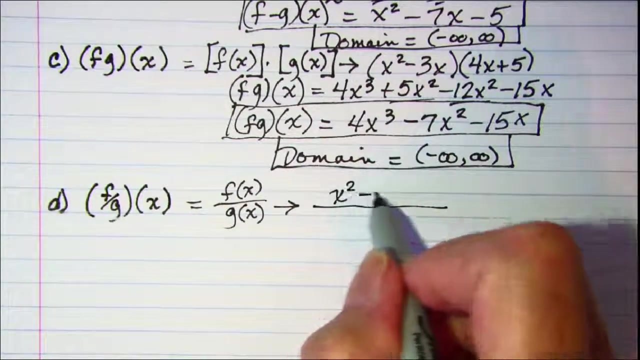 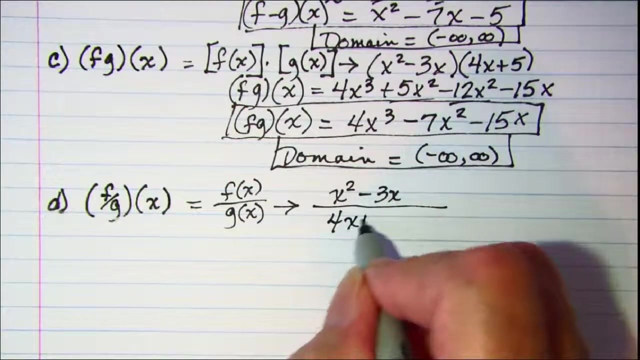 either domain. so my domain is all real numbers. Finally, let's look at f divided by g of x. This is f of x divided by g of x, which will be f of x in the numerator and x squared minus 3x and g of x is in the denominator, so 4x plus 5.. No, 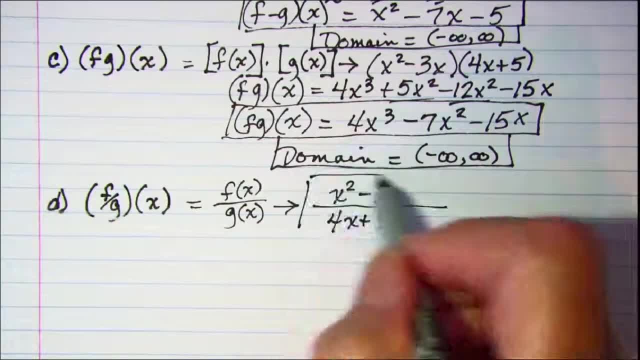 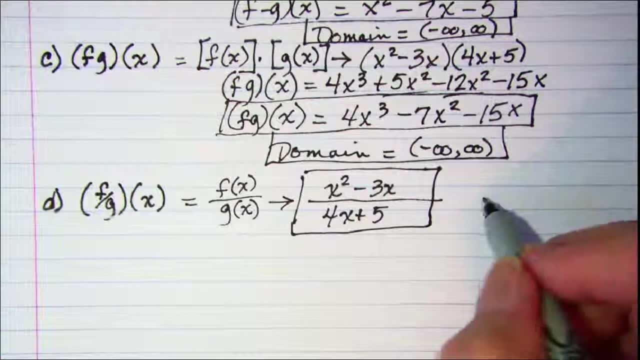 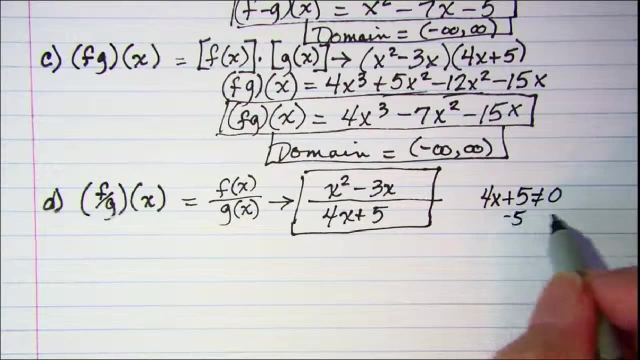 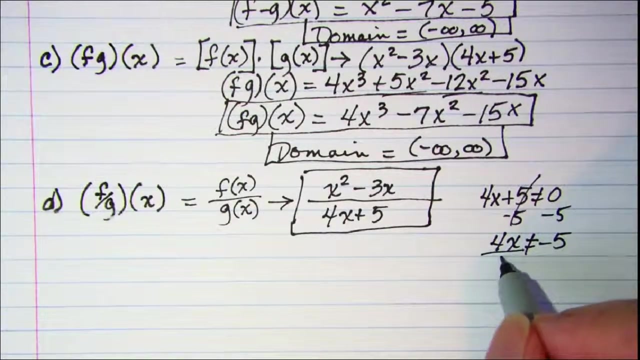 simplifying can be done here, but we need to designate that 4x plus 5 cannot equal 0. So subtract 5 from both sides, So 4x cannot equal negative 5.. Divide both sides by 4 and x cannot equal a negative 5. fourth, 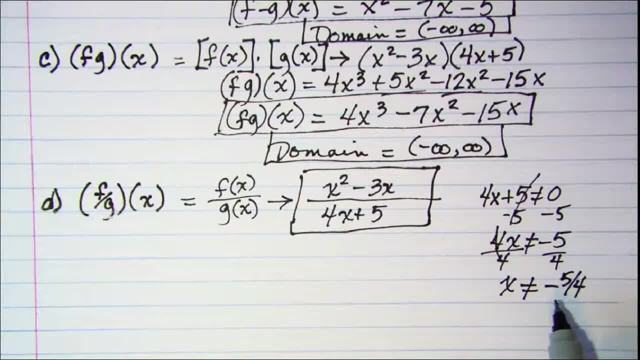 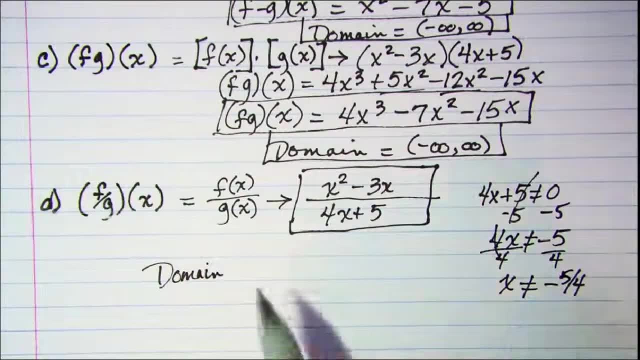 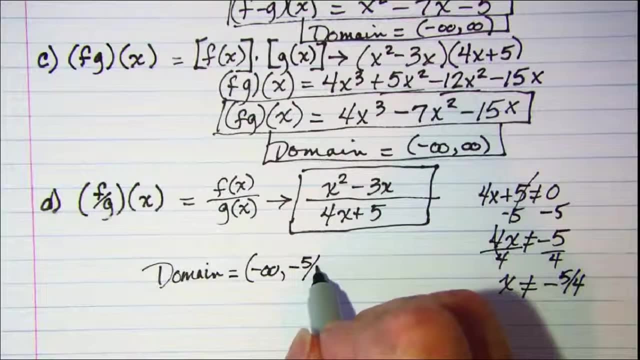 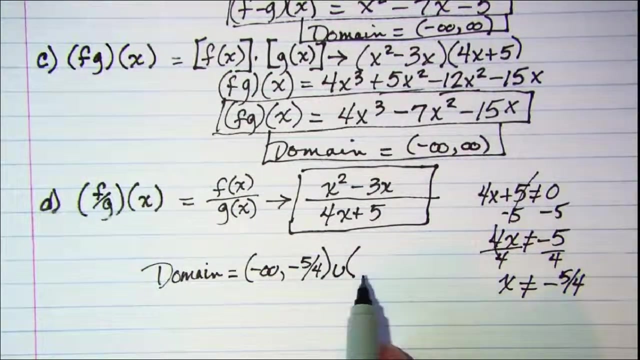 So our domain then, showing that in interval notation is from negative infinity to negative 5 fourth. We're not including this here, so we'll use this one from the denominator including that negative 5 fourths union width, and then we're going to pick up on the other. 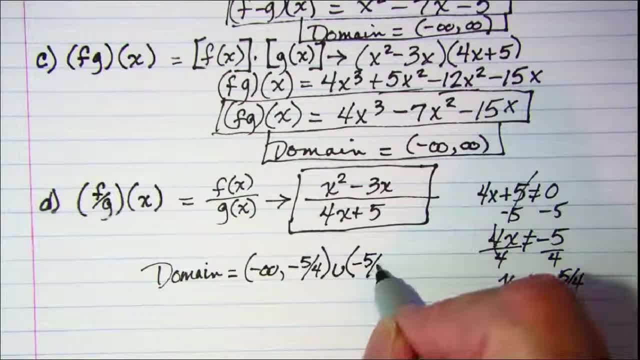 side of negative, 5 fourths and include all real numbers up to positive infinity.